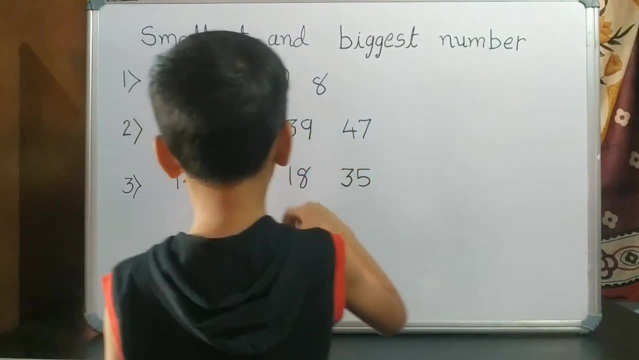 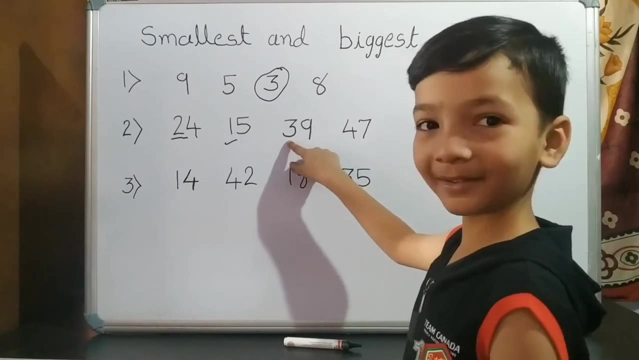 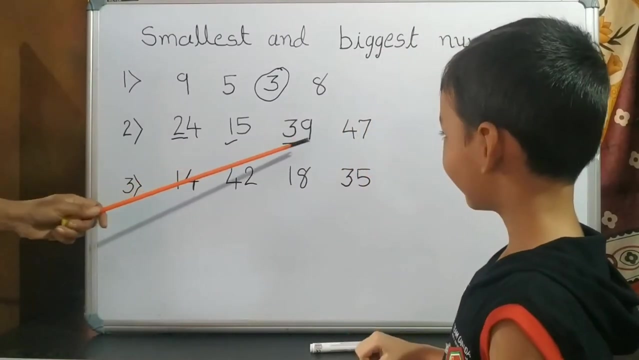 1. Which number is on 10th place of 39?? 3. Underline the number on 10th place of 39.. 2. Which number is on 10th place of 39?? 3, 2, 2, 2. 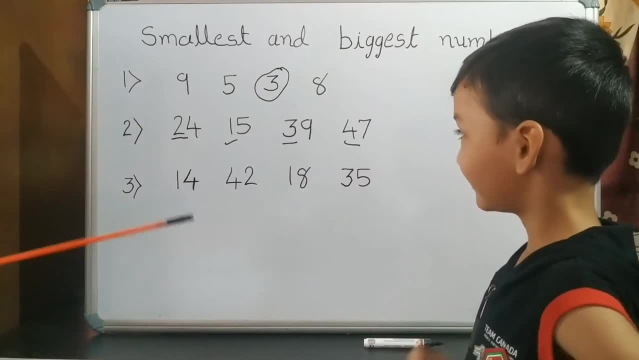 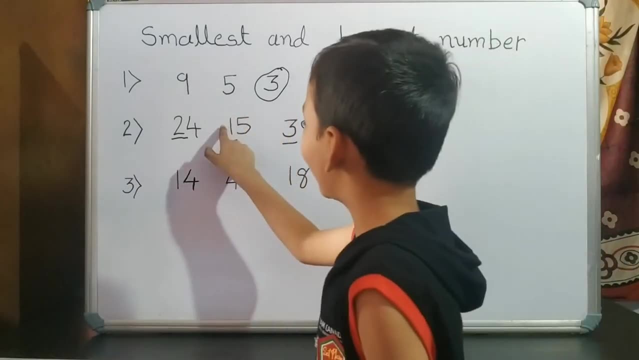 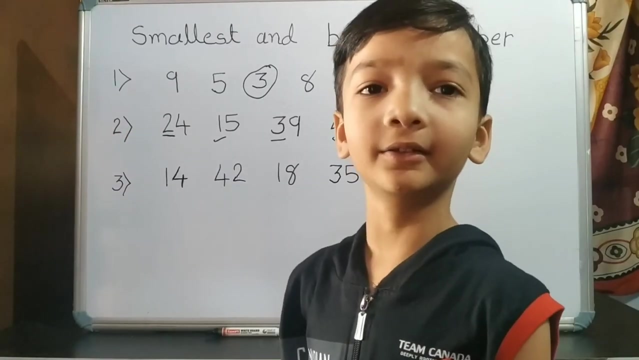 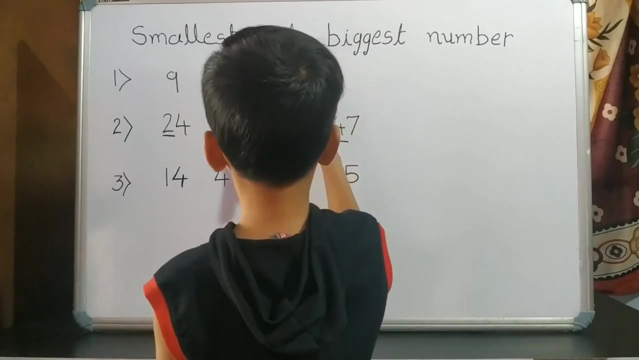 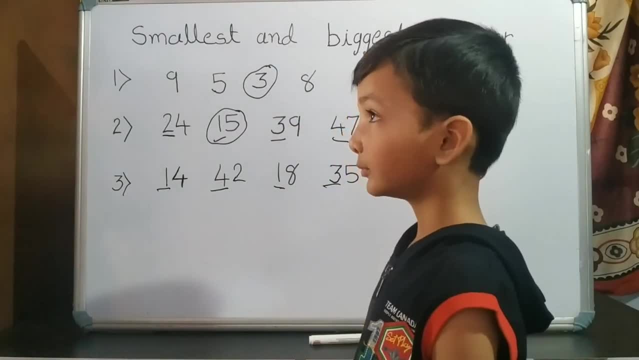 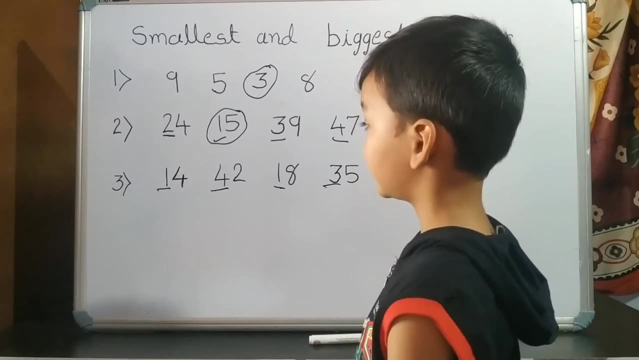 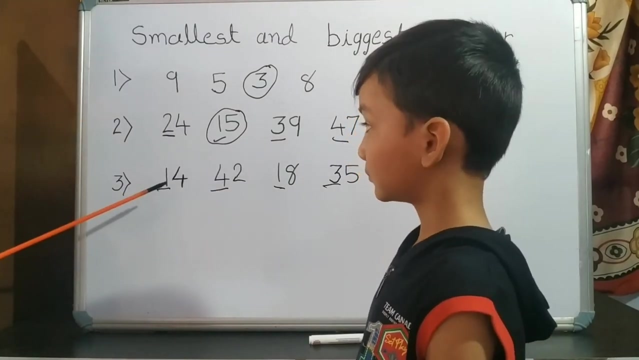 Very good, Now tell me which number is smallest on 10's place 1.. But we have two numbers which have number 1 on 10's place. So what we will do? We have to check numbers on 1's place. 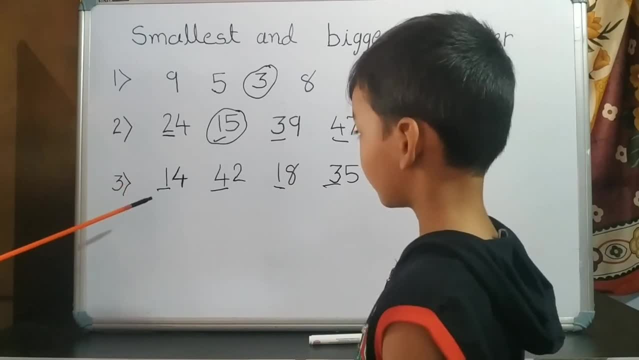 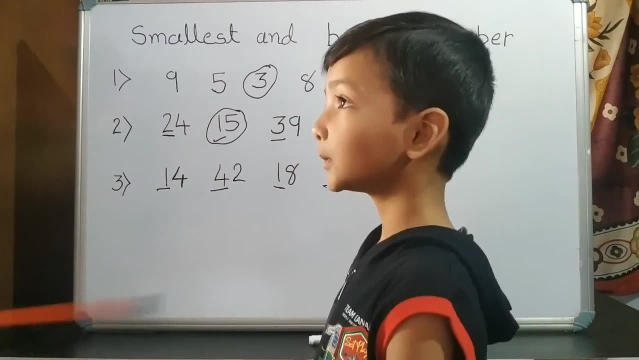 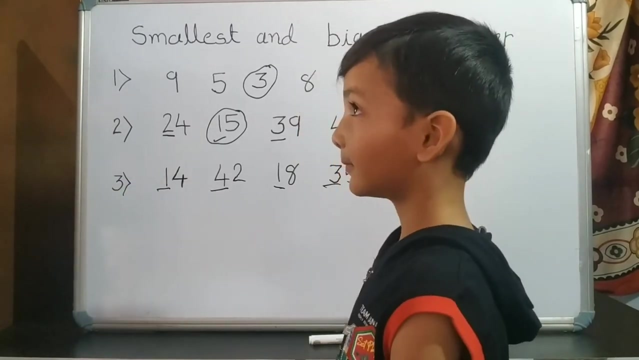 Now tell me numbers of 1's place of 14 and 18.. 4, 8.. Very good, Which is smaller number, 4 or 8? 4.. So our smallest number is 14.. Circle it. 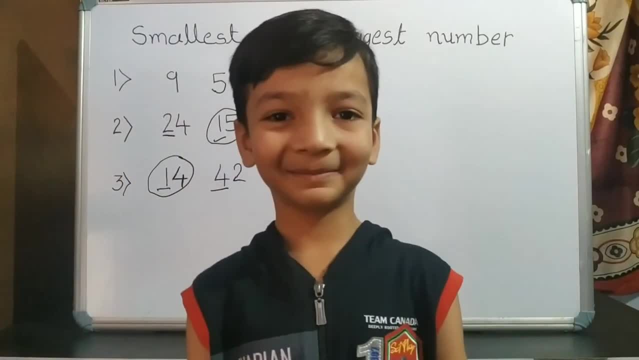 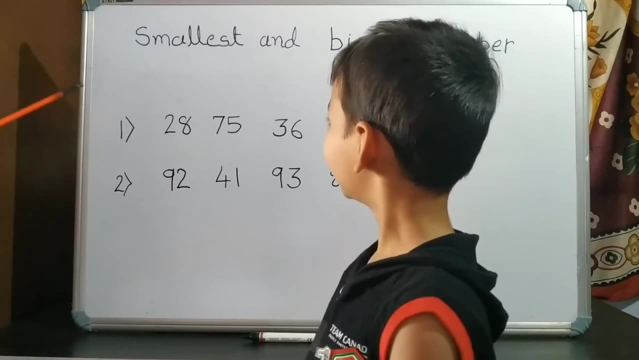 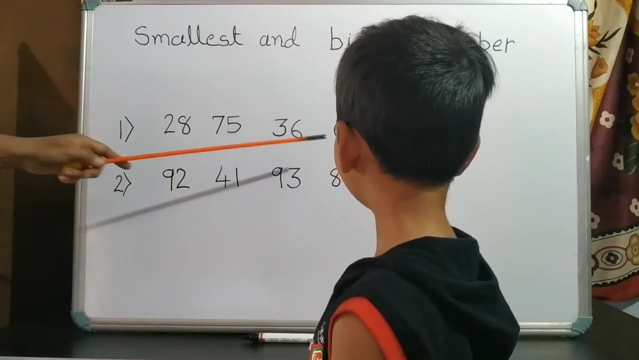 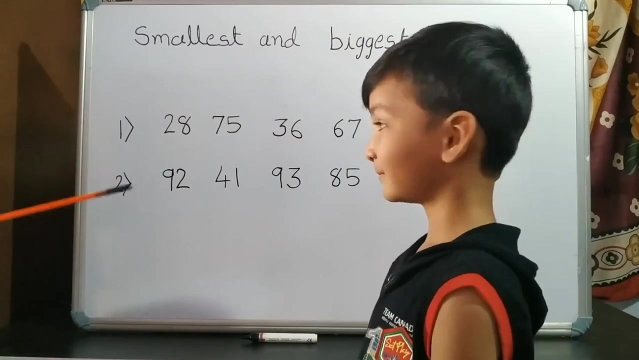 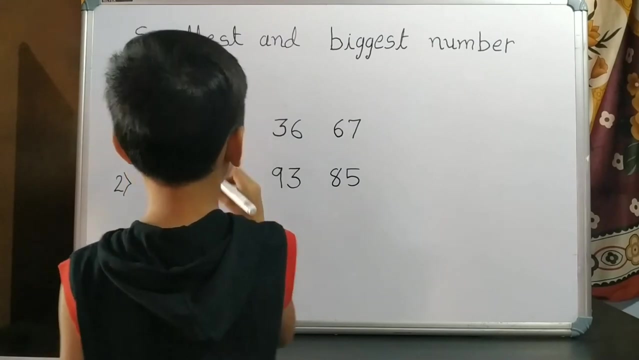 Excellent. Now we learn how to find the guess number. Here we have numbers 28,, 75,, 36,, 67.. Now underline all the numbers of 10's places: Yes, 2., 2,, 7,, 3,, 6..